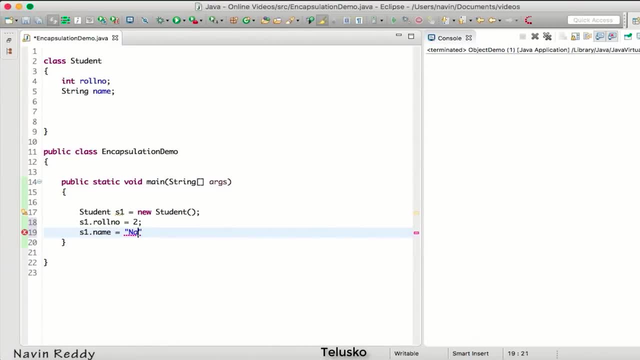 S1 dot name is equal to, let's say, Naveen. So when you have, so when you are assigning the value of S1, row number two, and Naveen. so we are trying to access that from main method. So it is. 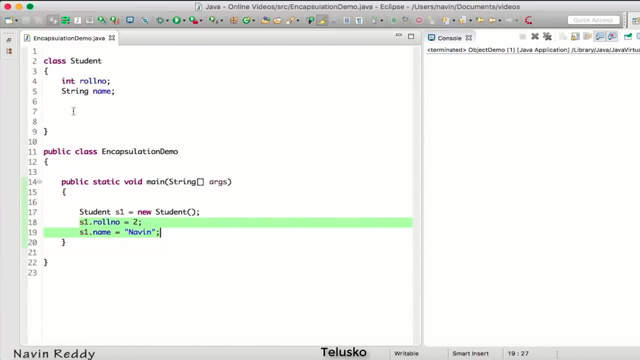 not right. So the only way to access the row number and name should be through methods. So normally those methods are basically called as getters and setters. You know what exactly it is. So to set the value, we have to use setters, and to get the value, we have to use getters. Example: 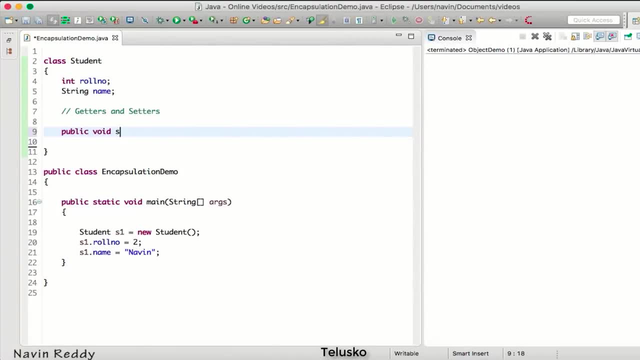 so let's say I want to set the value for row number. I will say public void. Since I want to set the value, I will use the method name as set row number. We have to make sure that is R is set row number. Or we can also say R And now I can say row number is equal to R. So we are. 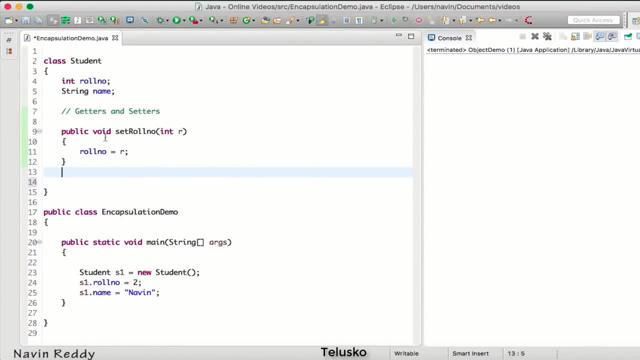 assigning the value of R to row number. That is one way How to fetch the value of row number. So we'll say public, Now, since we want to fetch, we'll return int and we'll say: get row number. And now this will not accept any value, right? But this will return a value. It will return a row. 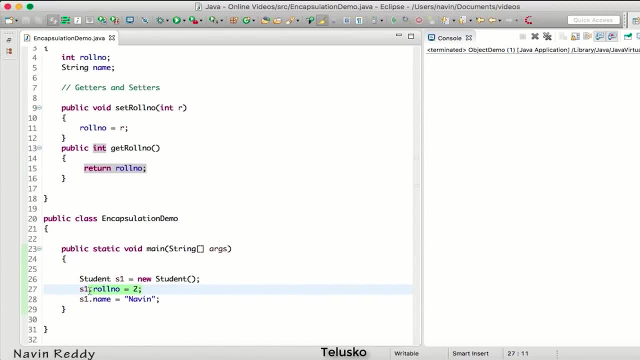 number. And now, if you want to access that, we have to say S1 dot- set row number. by specifying S1 dot- get row number. So we're not assigning the value directly, right, We're assigning the value through a method. That means the only way to use the variables is through a method And we 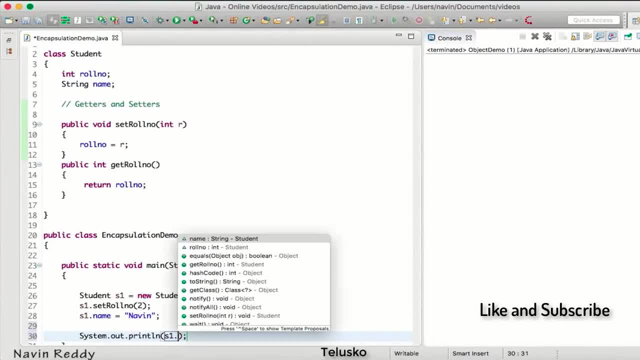 can also fetch it now. So let's say, let me fetch the value. I will say S1 dot get row number. So instead of saying S1 dot row number, I'm saying S1 dot get row number. And if I run this code, 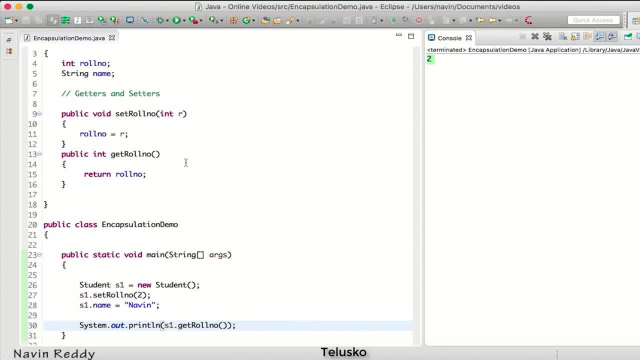 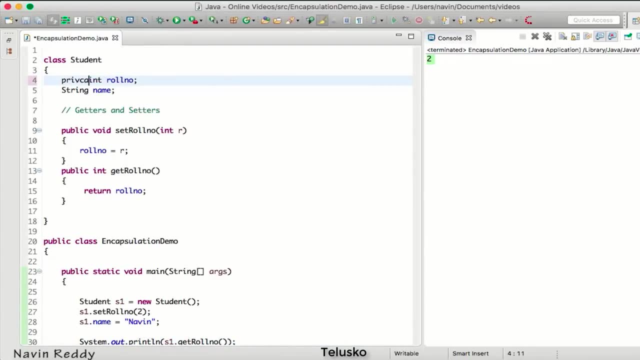 you can say it will work. So you got two. So the only way to access the variables is through methods. And since you're accessing the data through methods, we can also make this variables private. So you have to make sure that your variables are always private. So variables. 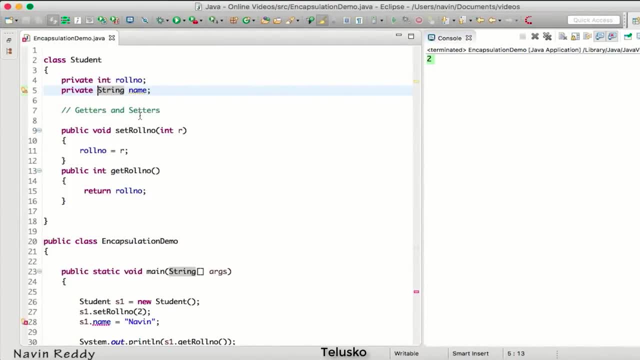 should be private And the methods- who will access those variables- should be public. That means you are binding your data with the methods And whenever you bind your data with methods, the concept is called as encapsulation. So the concept of encapsulation is it is binding data with. 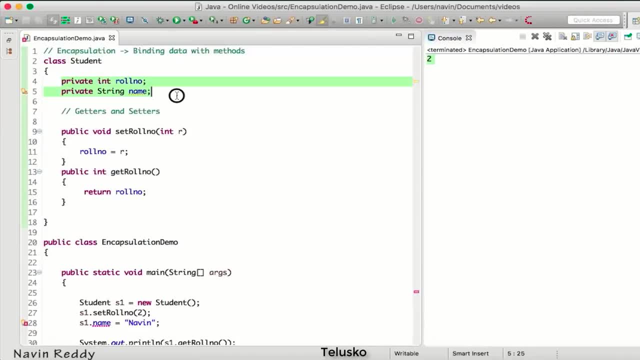 methods. So it's binding data with methods. So we have a data here and we have some methods here. So the only way to access the variables is through methods. But we have done that for row number, right. We have not done that for name. The thing is. 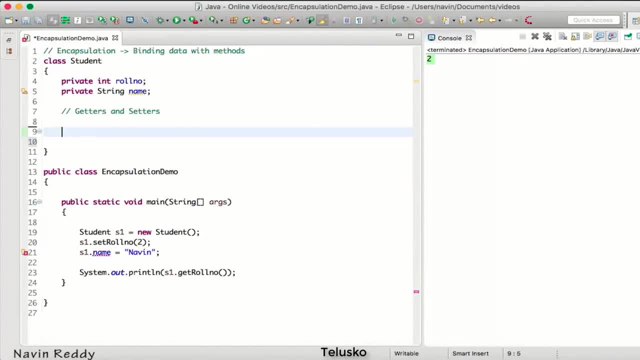 if I do this for names, I have to type it right. But encapsulation is so famous you just, you can simply ask your Eclipse to give it for you. So you just have to right click. you have to say source. 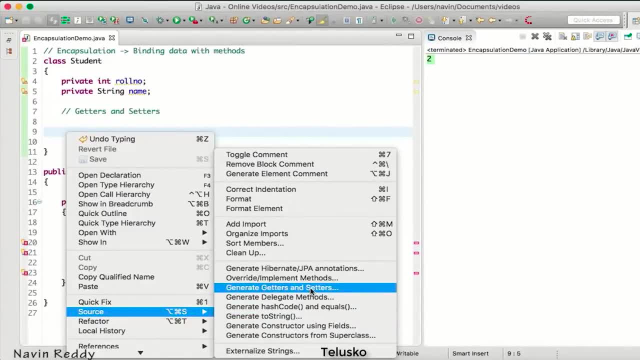 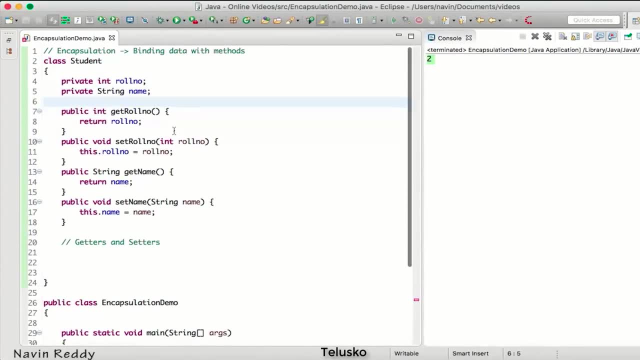 you have to click on generate getters and setters. Can you see that And select both the variables and click on OK, as we have seen the constructors, So you can see, it is giving you both the, both the methods here: get row number and set row number and get name and set. 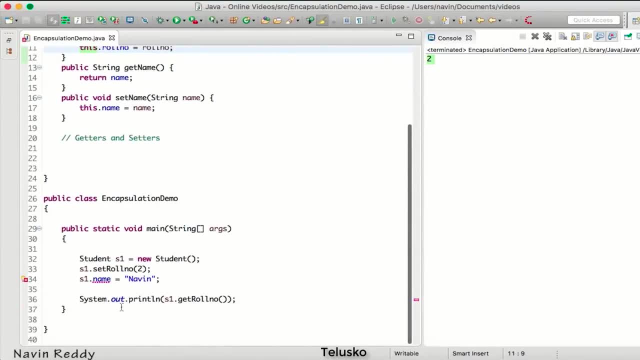 and we have also seen how to use this keyword, right, So you know about that. So, instead of assigning the value now, so you can see, we are getting error on this line because we have made name as private field, right. So if you see the, if you see this, it is giving you an error, which. 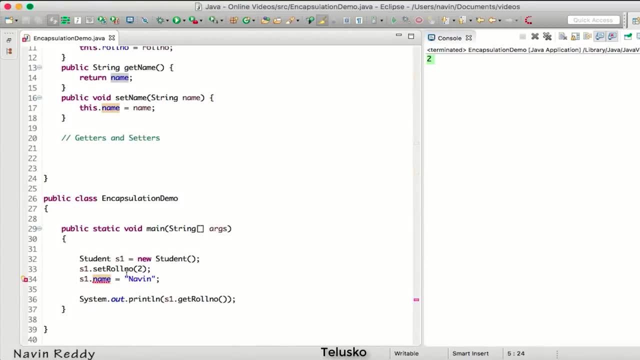 is student. dot name is not visible. So what we can do here is we cannot use name Now. we can say dot set name and we can pass the name there. So that that's how it works. If I run this code we got 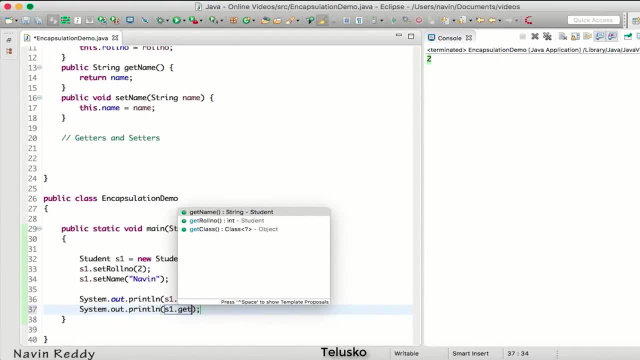 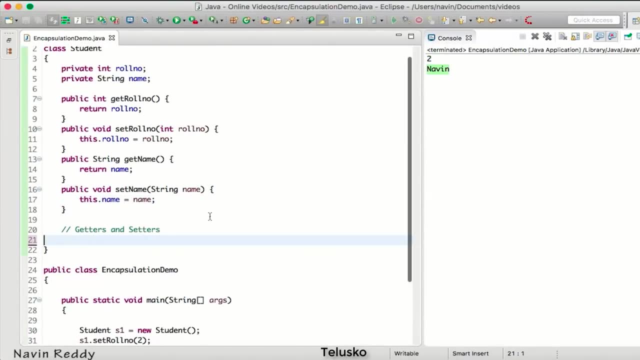 two, because we are printing only the row number. Let's also print the name. We'll say get name, And we got row number and name both. So this is, this is how you can use your getters and setters, and this is encapsulation. So that was the first part. The second part we have to talk about is why we 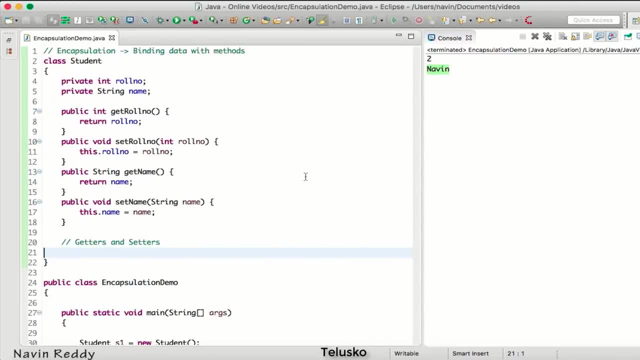 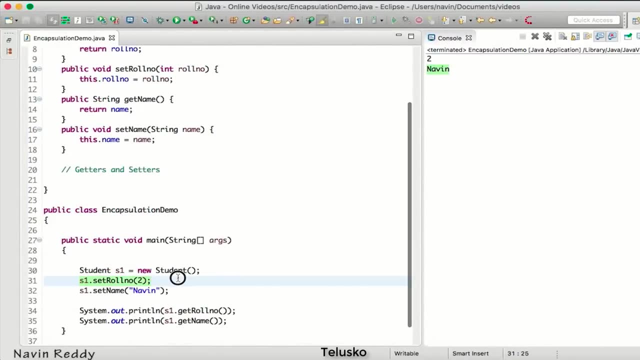 need it. The need for encapsulation is: we have to make sure that your data is safe, right? So this data needs to be safe. See if I want to assign the value, if you want to assign the value using to assign the value to row number, the only way is with the help of methods. right, We have to. 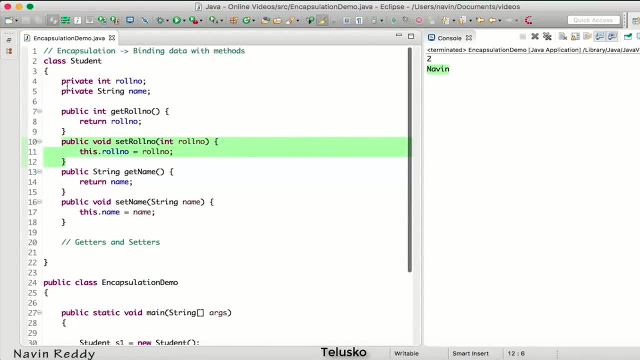 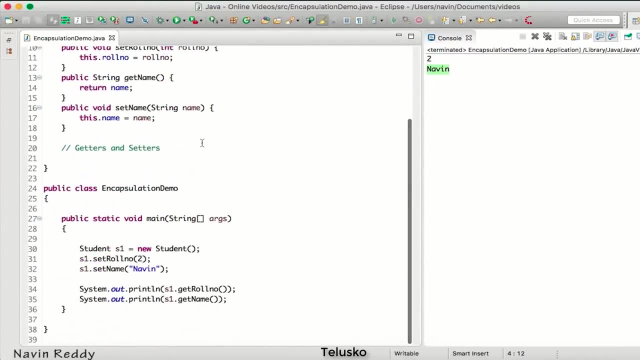 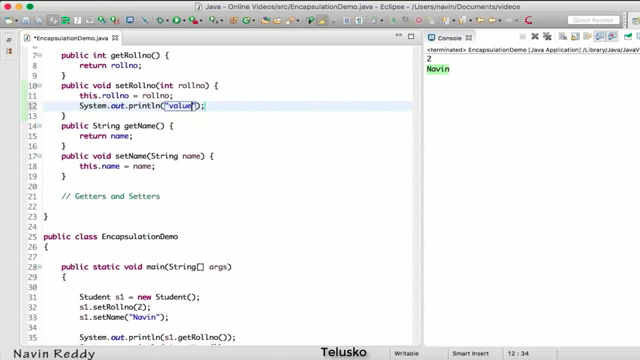 use set row number. Now let's say: if you make it, if you make this variable as public, anyone can access the variable right. What we want is, even if people are trying to change the value, I can simply print a log file. right, I will say: I can simply maintain a log file. We can say: value of: 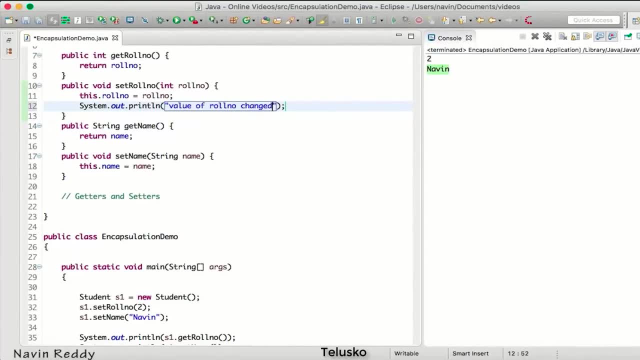 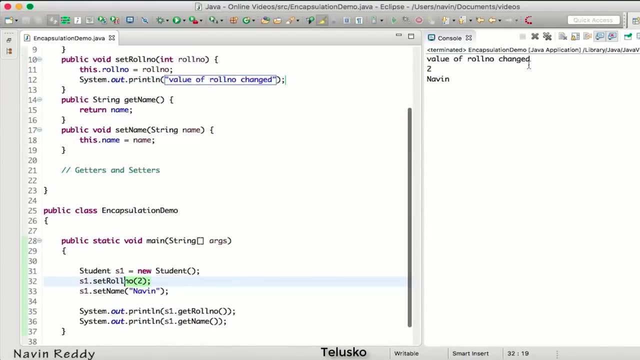 row number. row number change. I can maintain a log file, because when you talk about server level programming, we always maintain a log file. If you run this code now, it is assigning a new value, but it is also printing value of row number change. At least you can maintain a log file, So. 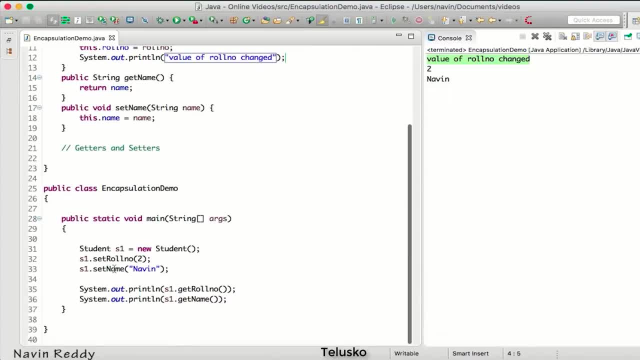 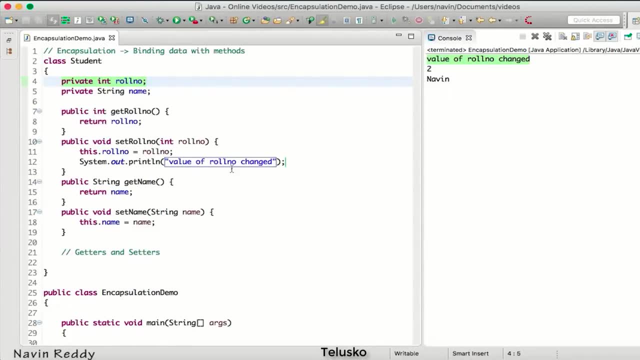 you cannot do that directly with variables. If I say s1.name equal to navin and if I have a public variable there, I mean how can I maintain a log file Changing the values of the variable or fetching the value of the variable? you can also maintain a log file that user has just fetched. 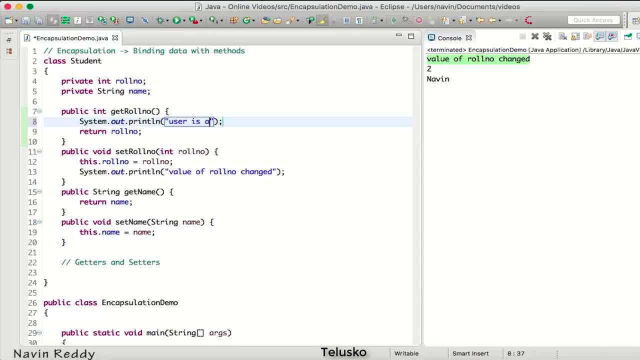 the value. We can simply say: user is accessing the value. At least it will maintain a log file for you. You can see that it is saying that user is accessing the value, So you can maintain a log file. Second use is: before fetching the value of row number, you can also check for the login of. 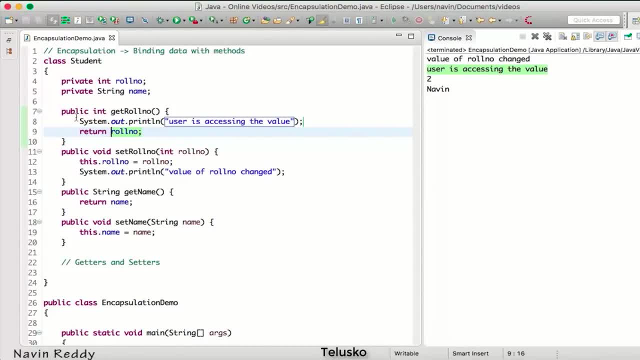 the user if user is already logged into the system, How can you do that? In this line, in this code, you can write those statements. So it's always better to access the variable with the help of methods, because that's the only way you should be able to access your variables. You have to make. 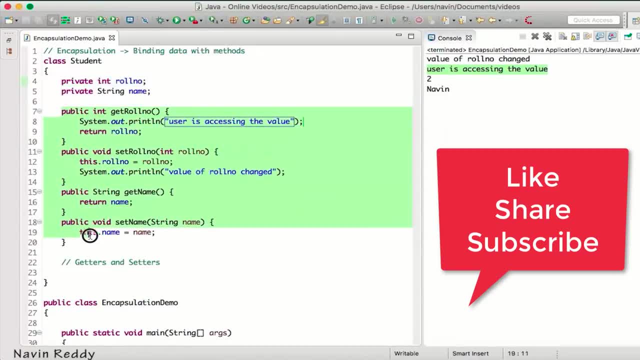 sure that your variables are private, and then you need to have a getters and setters who will access those variables. So that's it. That's about encapsulation. That's it about this video. 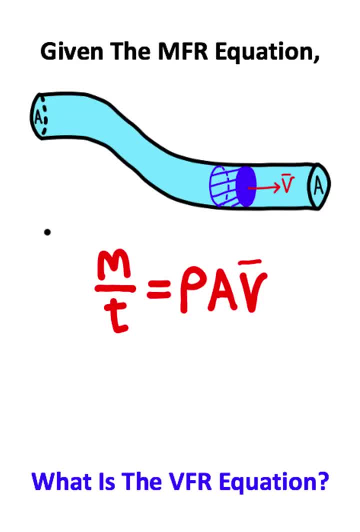 We have water flowing through a pipe and we are given the mass flow rate equation And what we want to do is derive the volume flow rate equation with reference to a small chunk of water that is flowing through the pipe. Now, because we are already given the 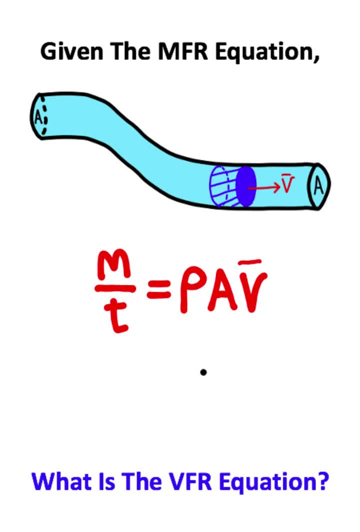 mass flow rate equation. the solution to this problem can be found pretty quickly. All you need to do is recognize that density is equal to mass divided by volume. This is always true for mass density, and if I use some quick algebra here, I can solve for the mass. So 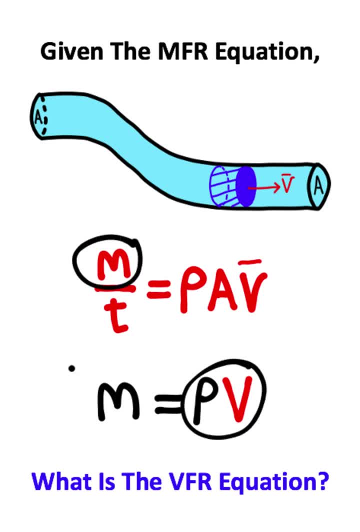 I can take the mass in the flow rate equation and replace it with density times volume. By doing this step, notice how the density cancels throughout this equation, leaving me with volume over time, which is the volume flow rate. So the volume flow rate is cross-sectional. 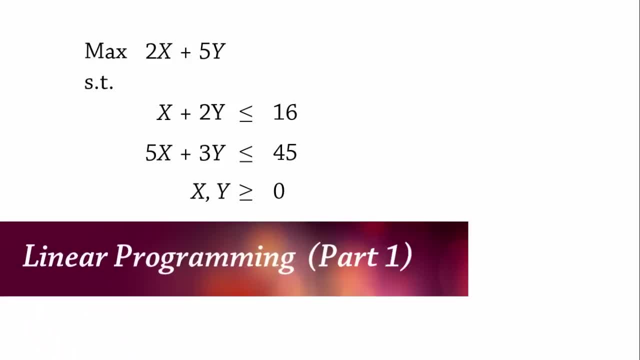 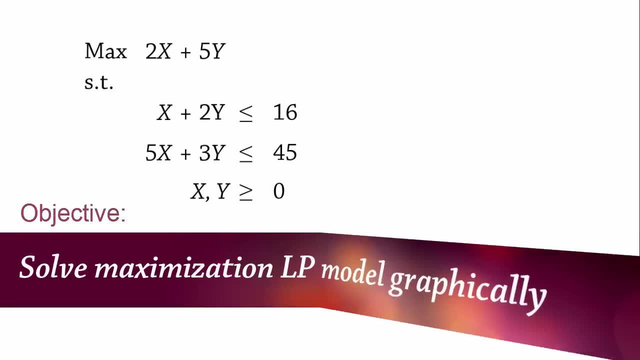 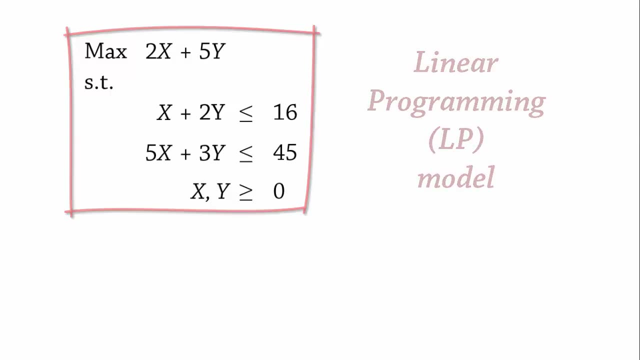 Welcome to the first video in this linear programming series. In this video we will graphically solve a basic maximization linear programming problem using the extreme or corner point approach. What we have here is a linear programming or LP model. The x and y in this model are referred to as decision variables. They tell us what quantity.